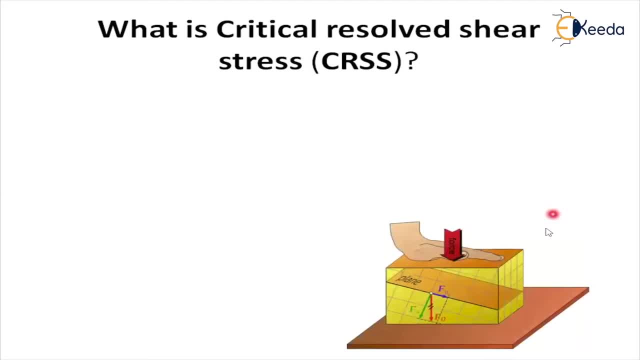 What is Critical Resolved Shear Stress? Just observe here: Here, if you apply a pressure on a material- maybe shear stress, So due to that it initiates slip, You can observe here It initiates slip. How much stress, that is, how much shear stress is required to initiate slip, is represented as Critical Resolved Shear Stress. 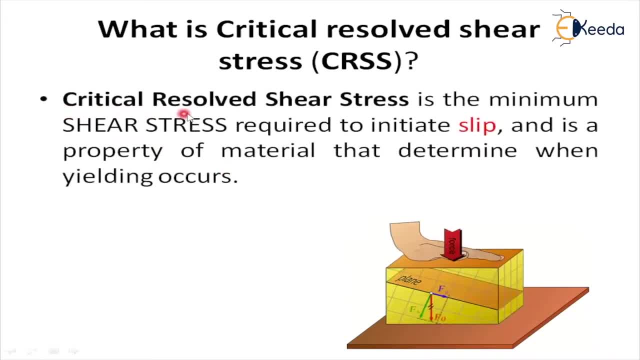 Observe the definition here: Critical Resolved Shear Stress is the minimum shear stress required to initiate slip and is a property of material that determines when yielding occurs. Here you are observing two points here. One is the shear stress required to initiate slip. If you observe the animation, how much shear stress is required to initiate? 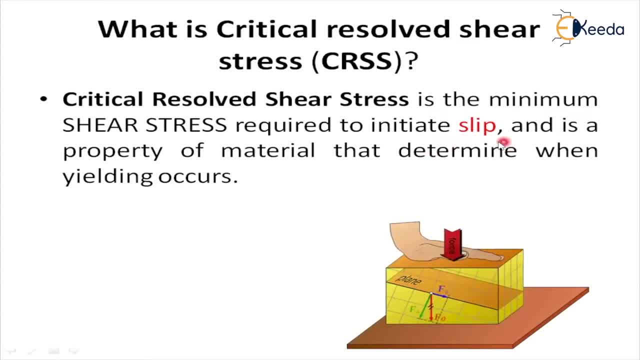 slip. That is a minimum. That is first point. Second point is this: critical resolve, shear stress, is a property of the material, like ductile nature of the material, like brittle nature of the material. Critical resolve, shear stress, is also a property of the material. 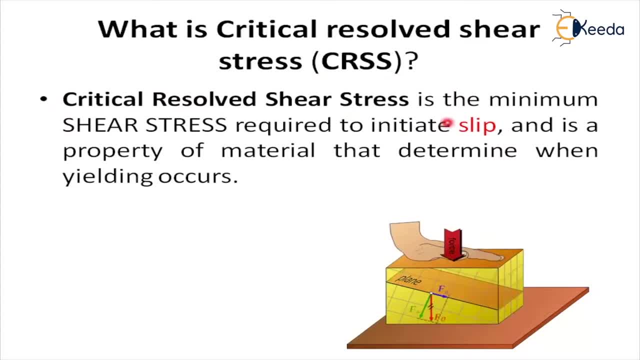 How it is property of the material we will discuss in coming slides. And one more point: we must understood that it is constant for given crystal. So that means for a particular material, the critical resolve, shear stress value is constant. Suppose for steel, CRSS is constant. 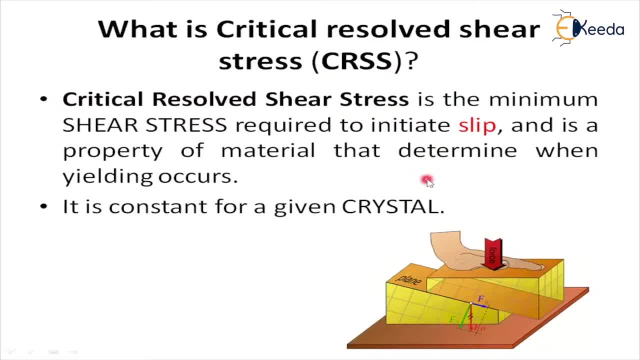 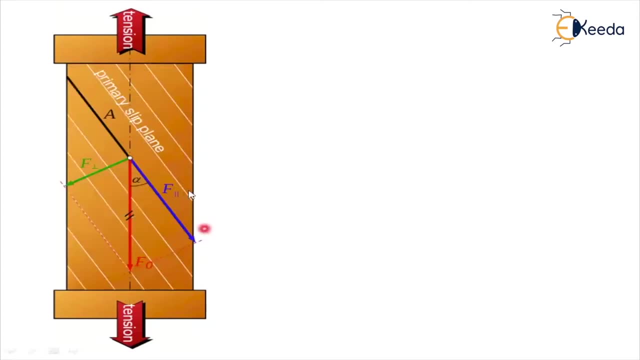 It is not depending on the force applied or any other thing. It is completely the property of the material. You can observe in images like this. Observe this image. This is a specimen In general, in initial stage, the specimen is represented as a slip plane here And the 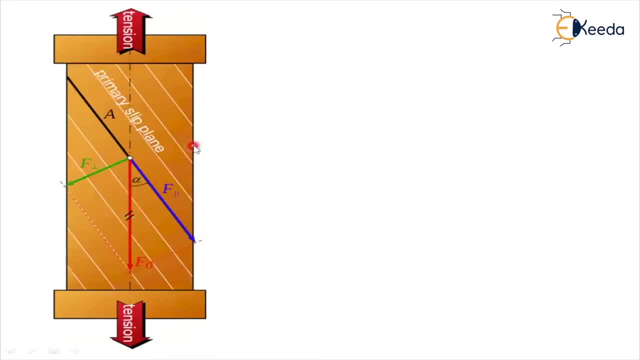 slip plane means if any force is applied, if it reaches to the minimum level, then this slip plane may disturb. How much force is required? That depends on the material. These are the slip planes. Depends on the tensile force or compressive force. These slip planes. 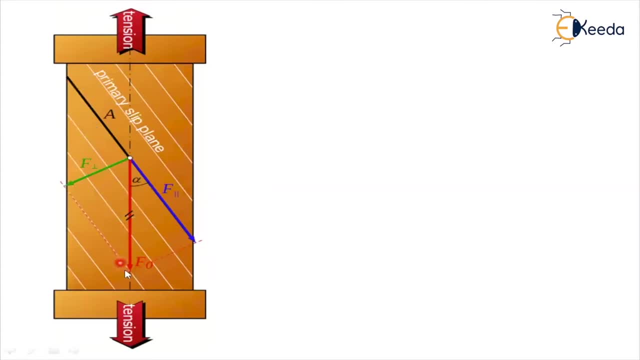 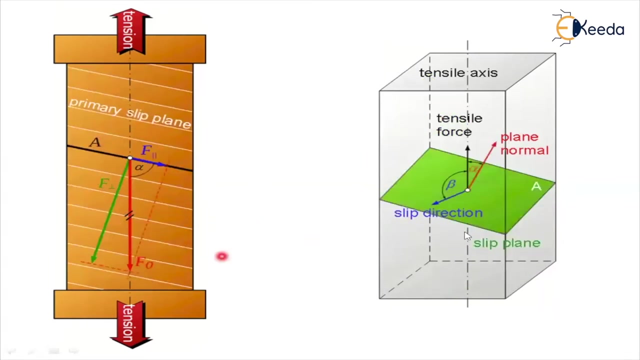 may be distorted from the regular axis. Here the slip plane will be the main part of the slip plane itself. You can observe in another image How the slip plane is changing the direction Here, in understanding critical, resolved shear stress, We must understand what do you mean by resolved? 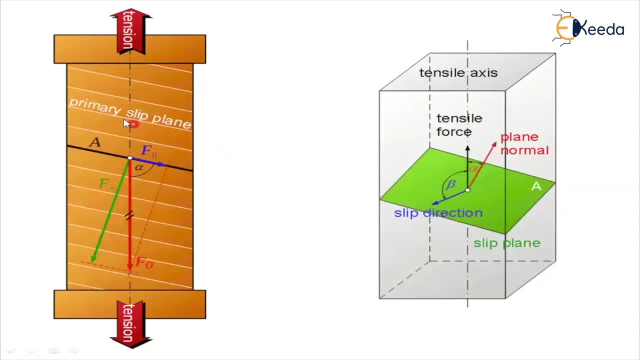 shear stress first. Here, if you observe, is the primary slip plane. here, in initial stage it is represented as a primary slip plane. When force is applied, the slip plane changes its direction. how much change is existed? so those things matters here. now let me explain. 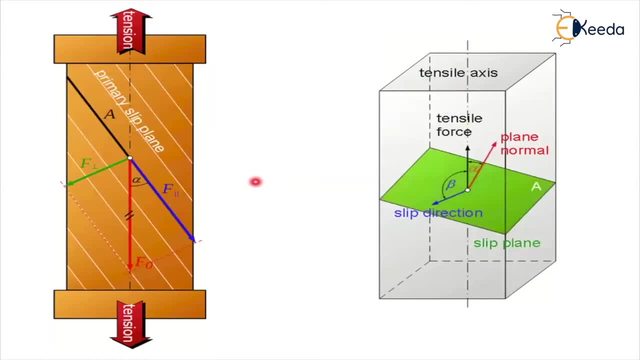 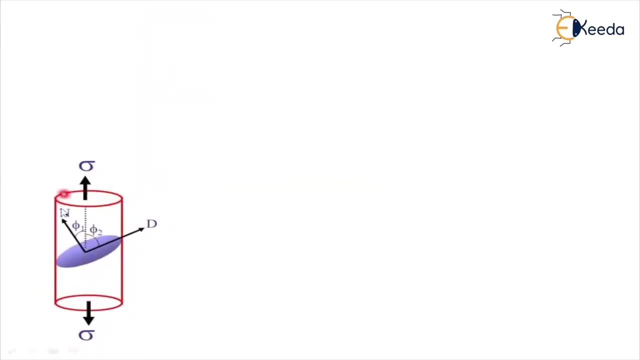 resolved shear stress in a material. let us take one specimen like this, and in that specimen let me explain what is resolved shear stress. now let us take a cylindrical specimen. a tensile force is applied here, like this sigma tensile force is applied. due to this tensile force, a slip plane may be existed. and here you are observing two directions here two. 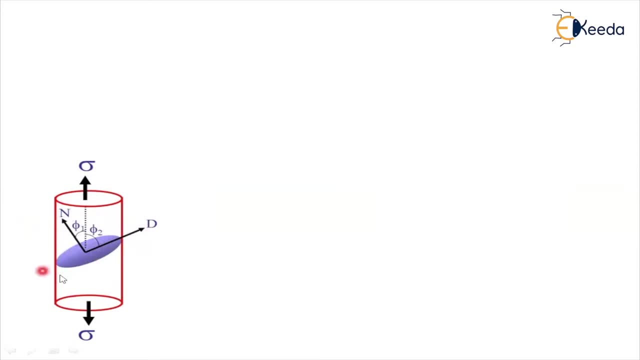 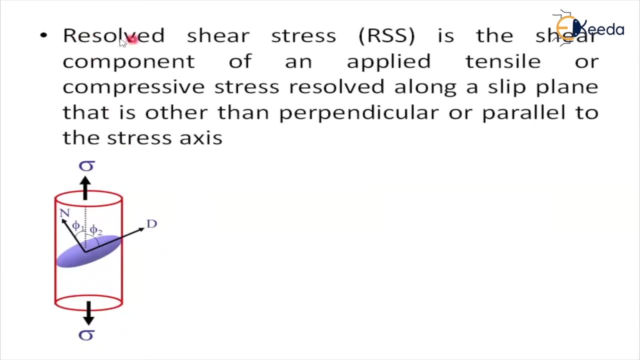 directions. let me explain in this what is resolved shear stress. please observe the definition first. the resolved shear stress is the shear component of an applied tensile or compressive stress, so means you can have the tensile force or compressive force- the result is same- compressive stress resolved along a slip plane that is other than perpendicular or 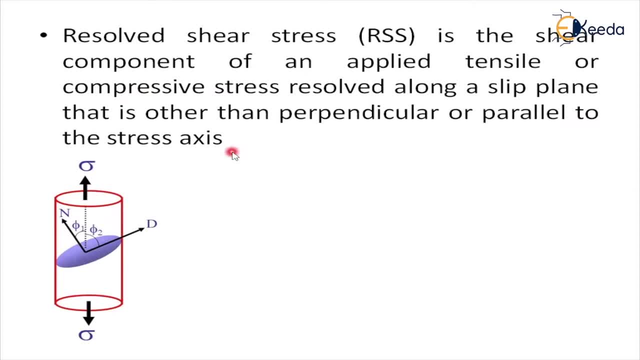 parallel to the stress accessor. so resolve stage. stress means here the direction is other than perpendicular or parallel to the force of rendre. thanks for your attention. stress axis. so that means here this is not the axis, here this is the resolved shear stress direction. now we have to concentrate the magnitude and the direction of the slip plane, suppose if 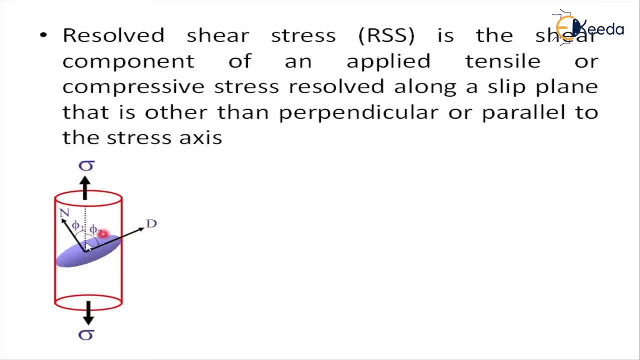 because of this tensile force. if this slip plane moves automatically, the total specimen may have some deformation due to that deformation. if you able to identify the deformation and the magnitude of the deformation, we can easily assess how much deformation may be observed for a particular tensile value. so this is very, very important parameter in understanding deformation. 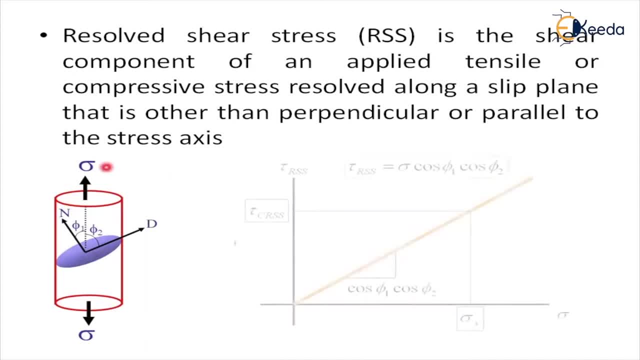 and material properties. now you can observe the same critical resolved shear stress. that is, resolved shear stress first, and then we have to concentrate the magnitude of the deformation and the direction in a graph. this graph is between resolved shear stress versus stress. here this is the direction you can observe a straight line, here the slip direction. here slip plane direction is the slip. 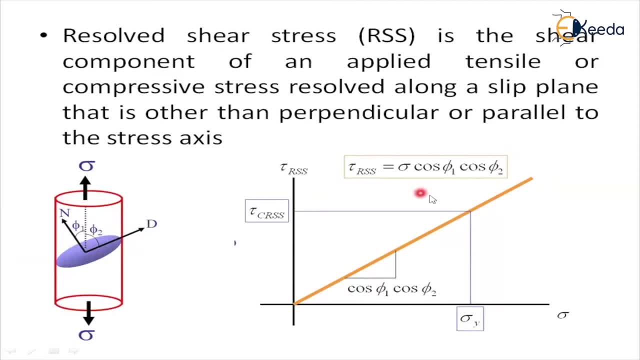 plane direction and the value. here you can observe the resolved shear stress is represented as: the magnitude of the resolved shear stress is sigma into cos pi 1 and cos pi 2. here what is pi 1 and what is pi 2 and what is sigma? here we will. 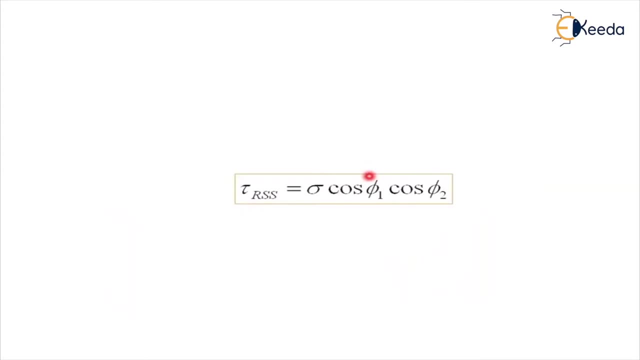 discuss. this is the magnitude of resolved shear stress. here one important factor we have to understand, that is skimmed factor. what is skimmed factor here? here the resolved shear stress is related to the applied stress by geometrical factor m, typically the skimmed factor. so that is cos pi 1 and cos pi 2. so means here you can observe this, cos pi 1 into cos pi 2. this magnitude is represented as m value here. m means here skimmed factor and it is multiplied with a sigma is denoted as resolved shear stress. 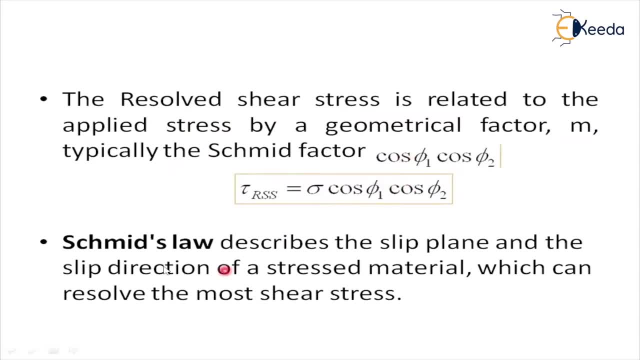 stressor. What is that law? What is Smith's law? The law describes the slip plane and the slip direction of a stressed material which can resolve the most shear stress. So these two angles are very, very important. According to this law, if these two angles are sufficient or minimum value. 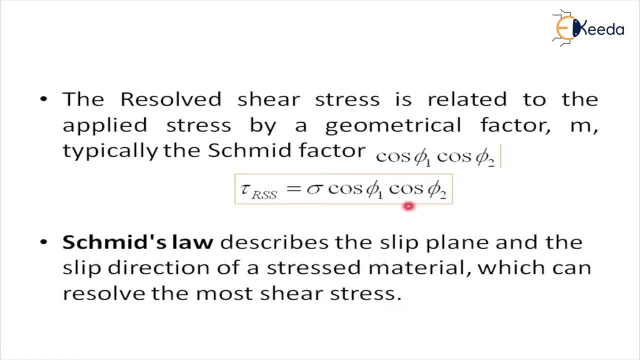 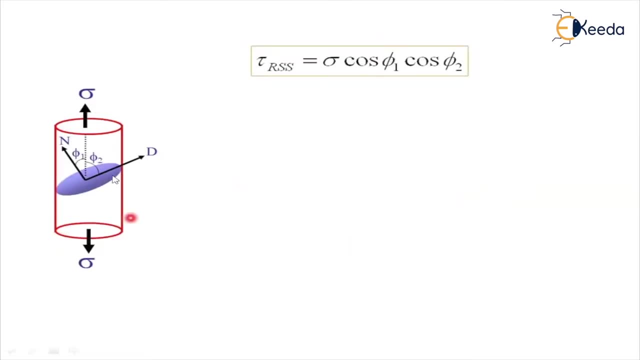 then automatically the slip plane may disturb the particular material. Let us discuss one more point here, that is, what is sigma and what is pi 1 and what is pi 2 here? Now observe the specimen here. In this specimen you can observe the pi 1, pi 2 and sigma. Now what is sigma here? The sigma. 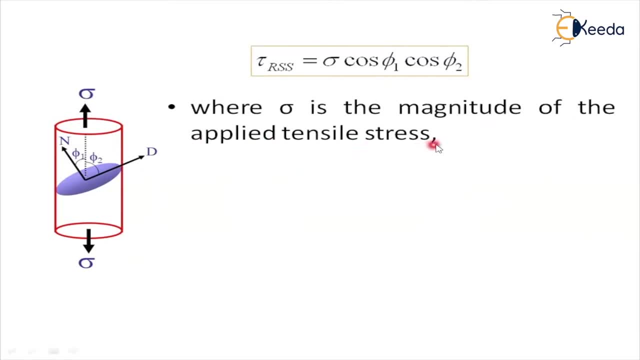 is: magnitude of the upturn. Applied tensile stress, Magnitude of the applied tensile stress. That means how much tensile stress is applied on the specimen. The next one is pi 1. here You can observe the pi 1 angle, This angle. 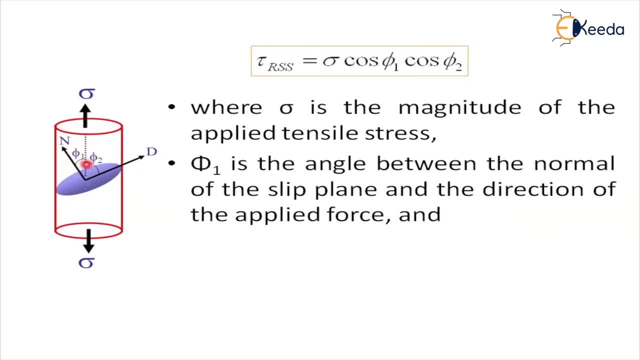 is between the normal- This is the normal- of the slip plane. This is the normal, This is the axis Normal of the slip plane- and the direction of the applied force. So this is the direction of the applied force. Pi 2 is the angle between the slip direction. The slip direction is the slope direction. 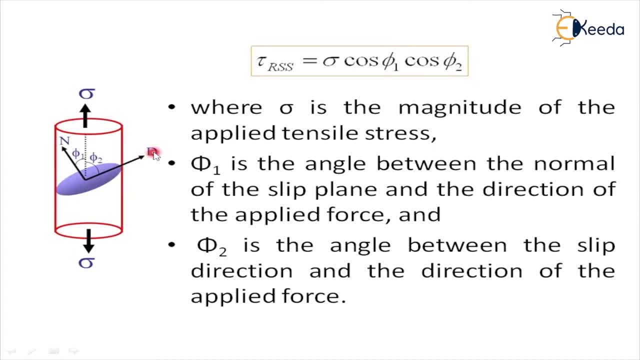 it is represented as D here. This the slip direction, The angle between the slip direction and the direction of the applied force. So this is the direction of apply force, and the angle between direction of the applied force and the slip direction is represented as pi 2.. Now, if you, multiply cos pi 1 and cos pi 2, it is a actual lost of energy. As you can see, this is what we call as a fission process. At this distance between the slip blade, the vector is recognized as needed. So we want to. 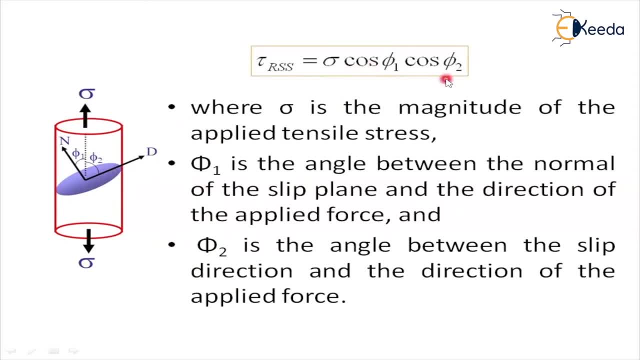 pi 2, it is represented as skimmed factor. and if it is multiplied with the sigma, that is the magnitude of the applied tensile stress, it is represented as resolved shear stress. Now, after knowing all these things, we must have some more salient features about skimmed. 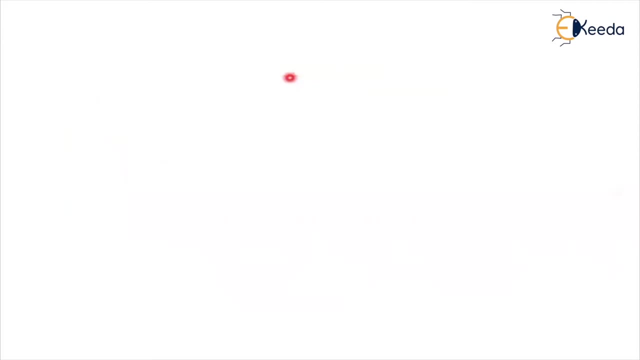 factor. So what is skimmed factor here? Please observe one more salient feature. Just observe the sentence: the skimmed factor is most applicable to FCC single crystalline metals. So that means most of the FCC metals are having this type of nature, and you can observe in another. 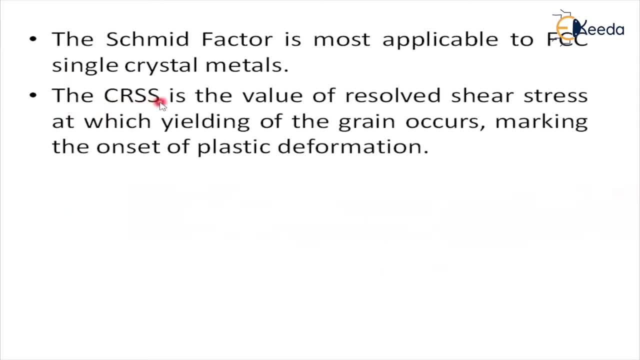 sentence. the critical resolved shear stress is the value of the resolved shear stress at which yielding of the grain occurs, marking the onset of the plastic deformation. What it means, Please observe the sentence. In initial stage the stress is directly proportional to strain. Nothing happens. But after that. 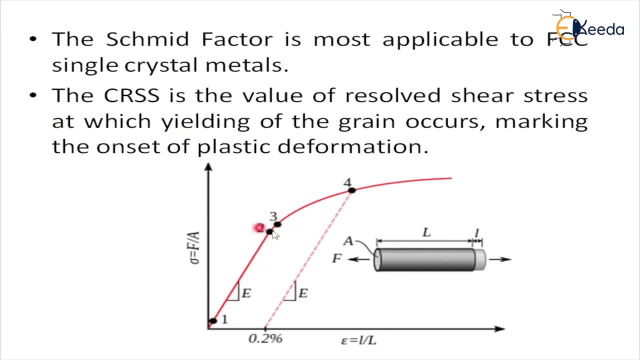 the yielding of. when it reaches to the yielding, then the plastic region starts here the minimum value: how much minimum value is required to disturb, to deform the material? So the value, that value is independent for the material to material. so that means it vary from material to material. So here the critical resolved, shear stress is the property of the material. 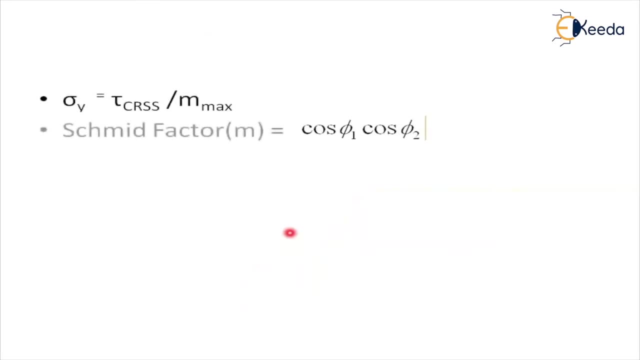 What is that value here? Please observe these two things here. First one is: sigma y means yield stress. So yield stress is equal to, is represented as critical resolved stress value divided by The m means the stress of the material, So the stress of the material, So the stress of. 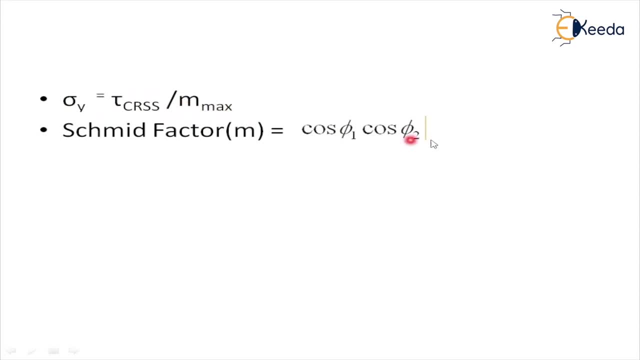 the material. The m means given factor, that is, cos pi 1 and cos pi 2.. The maximum value of skin factor. If this is the case, then this formula clearly shows that critical resolved shear stress is a material property and is not dependent on the applied lower or grain. 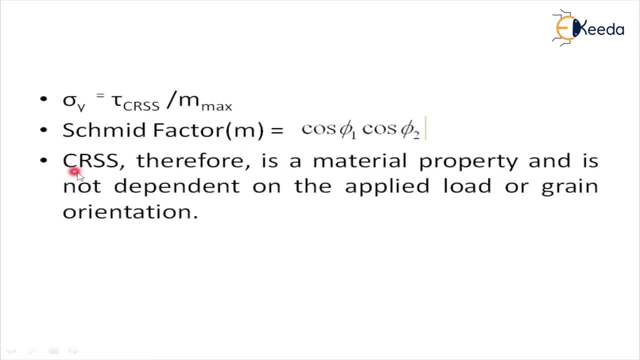 orientation. You can observe the sentence here. This critical resolved stress is not a dependent property. The m means given factor, that is, cos pi 1 and cos pi 2.. The maximum value of skin factor, So the stresses with respect to status, So 22 m times the yards. It is a material property. 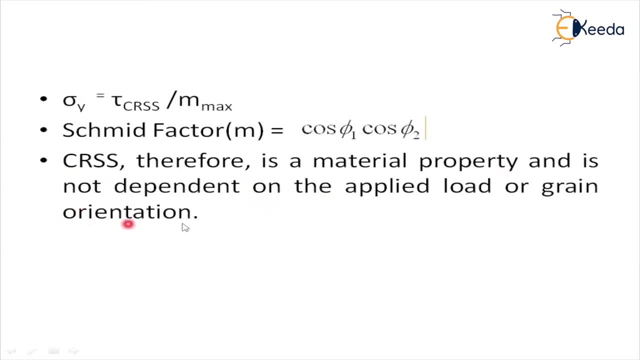 here. And one more salient feature regarding CRSS is that critical resolved stress is is related to the absurd yield strength of the material. So that means depends on the yield strength. suppose if the yield strength increases, critical resolved stress also increases. That is very, very important. So that means the critical resolved stress is directly incenseness. 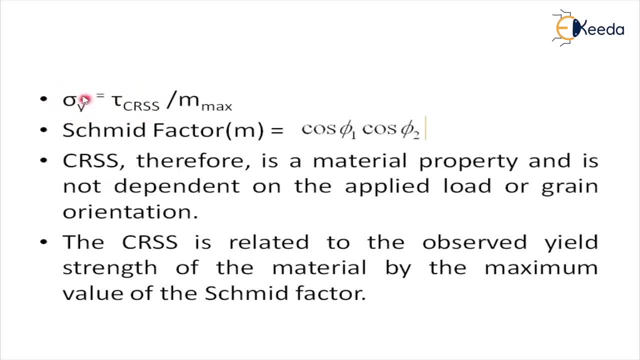 So that means that the salt is highabo posturemo, the burden of insertion is highand the function of this stress is that of large area shown here. The amount of flow have to be just, you guys, proportional to the yield strength of the material. So in another word, we can say that it is the property of the material, like ductile property or brittle property. Critical, resolved shear stress is also a property of the material.